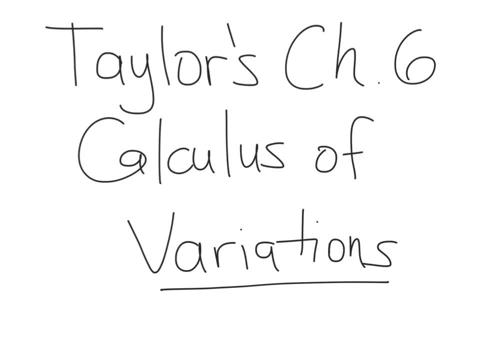 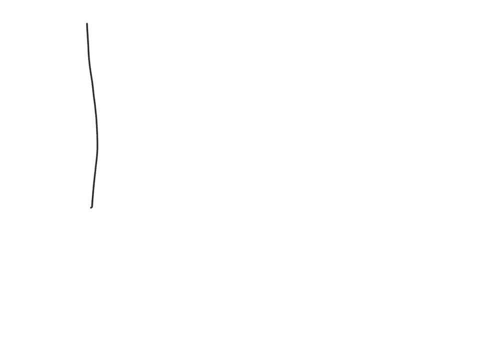 excuse me, Lagrangian mechanics to solve even the dynamics of very complicated systems. A nice example of a place where we can use the calculus of variations is to study the shortest path between two points. So let's think about an X and Y coordinate system. 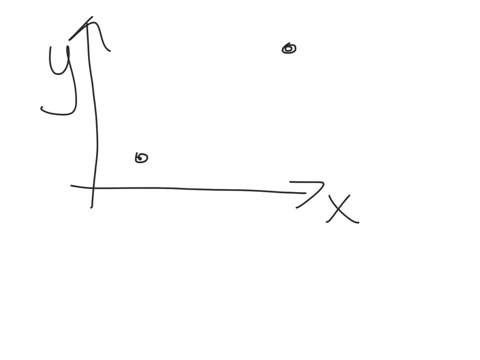 Let's imagine we have Y, One point and another point 0.1, 0.2. And we're interested in solving for the shortest path between those two points. Now, of course, we all know intuitively that the shortest path is going to end up being a straight line. in a two-dimensional space like this, 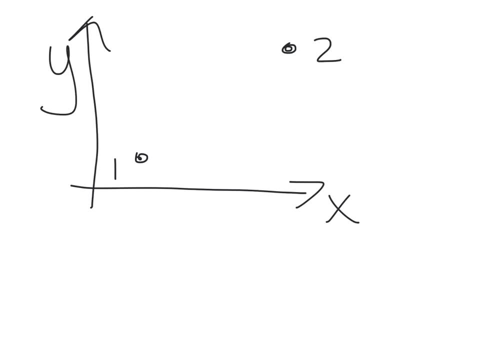 But how would we prove that? Well, calculus of variations provides us a way to do that. So let's start by considering an arbitrary line. So this is a path that's arbitrarily connected to the two points. Let's imagine that we've written the equation for this line. 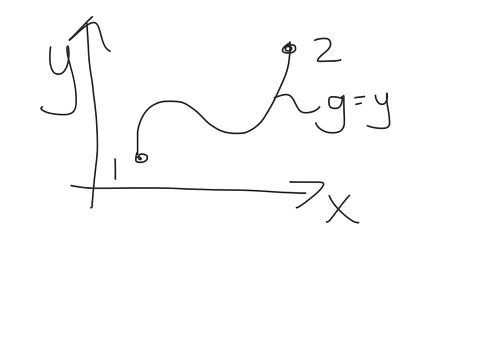 Y is a function of X. So here's Y, and Y is going to be a function of X, meaning, give me an X coordinate, I can tell you what the Y coordinate is. Now, as you recall, the arc length, a little bit of arc length along the trajectory that can be written as dS. 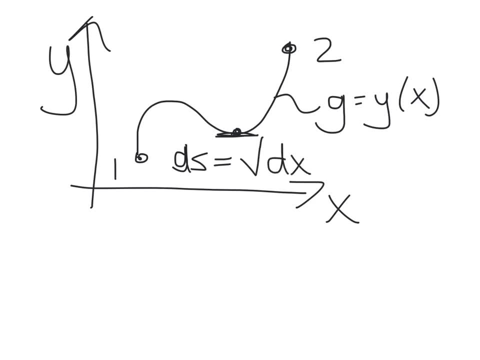 And then we've seen before that you can write dS in this way, so that it's the sum of the square of two differentials, dx, dy, and then the square root of all of that. Now, if I divide this equation through- excuse me, divide the radical through by dx, what we find is we get an equation for dS that has the X derivative of Y inside the radical times, dx. 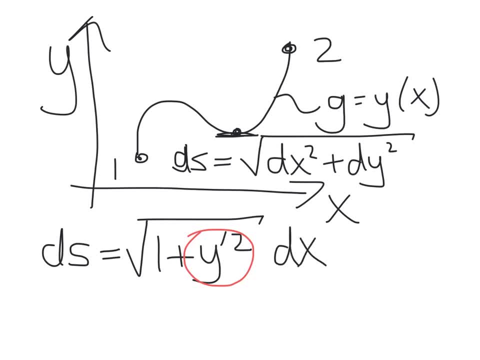 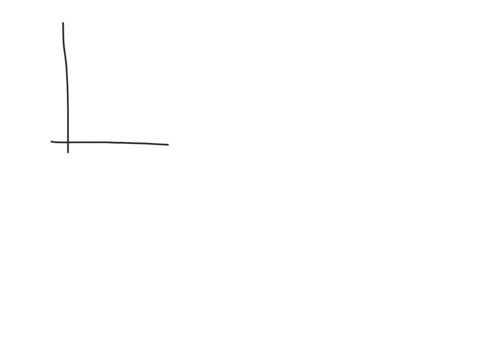 So that's a little bitty arc length. Now, if we want to calculate The whole length of our line, what we really need to do is to integrate that line, that dS, over the entire length of the line. So we're going to do an integral from 0.1 to 0.2,, 1,, 2, of dS. 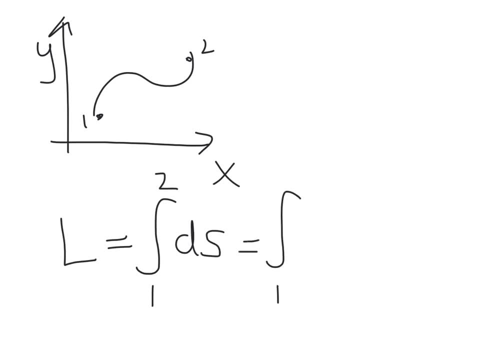 And so, using our previous expression for dS, we find that that total length of that line is going to be the integral of that square root business. So that's again the X derivative of Y dx. So we're basically trying to integrate this thing. 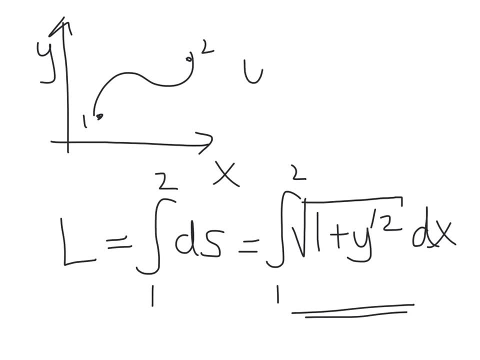 And what we want to show is that when we choose the right path, Y as a function of X, we will minimize this integral. So we want to choose the right path such that we minimize this integral. Now, as you might expect, it's not obvious. 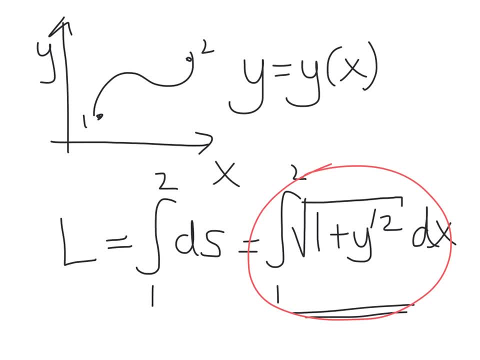 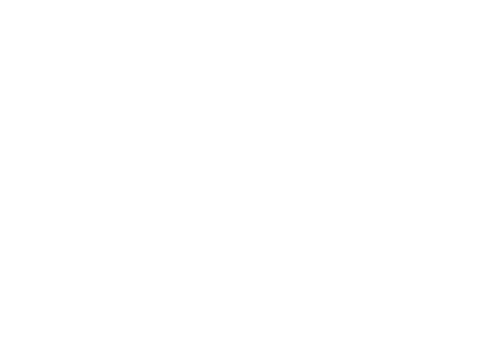 It's how you can actually choose the right function Y to minimize an integral. But the calculus of variation provides us a way to do that. Another physical problem in which we're interested in minimizing an integral is Fermat's principle. And so, for Fermat's principle, what we have is we might have two media with two different indices of refraction. 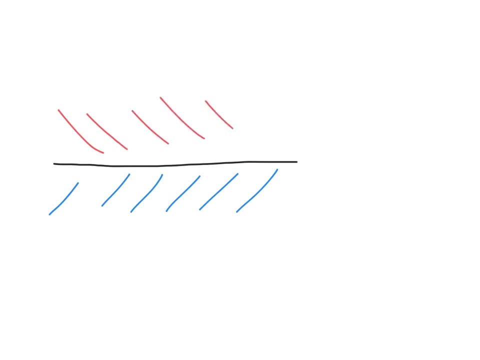 So here we're going to imagine there's two media, each with a different index of refraction, And we're interested in what path a light ray takes as it passes through these two different media. Fermat's principle tells us that the light will take whatever path produces a stationary value for the time traveled from one point to the other. 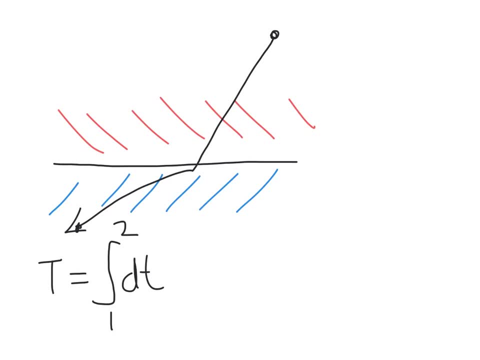 So what that means is we want to find a maximum or minimum value for the total time traveled by a light ray in going from one point to the other. Now, the time that it takes for a light ray to travel from one point to the other, that's an integral over dt the time. 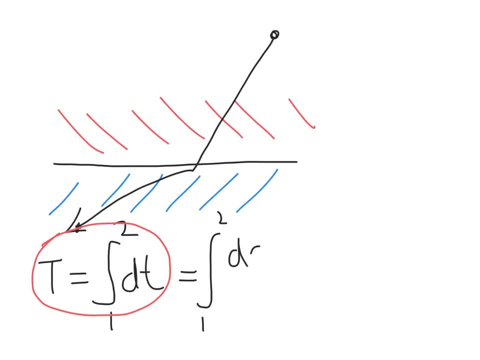 And, of course, dt. we can write that as a little length along the path ds divided through by the velocity of the light. Now, of course, the velocity of light is a constant in a vacuum, but it's not a constant when the index of refraction changes. 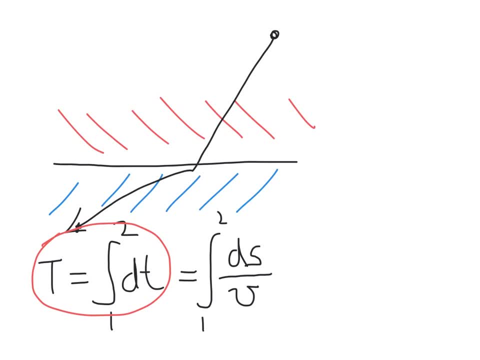 And you may recall that you can write the velocity of light in a medium using an index of refraction. So here, for example, this is the speed of light c in a vacuum And the velocity of light as it travels through these different media. that's given by n, the index of refraction, which can be a function of position in our system.